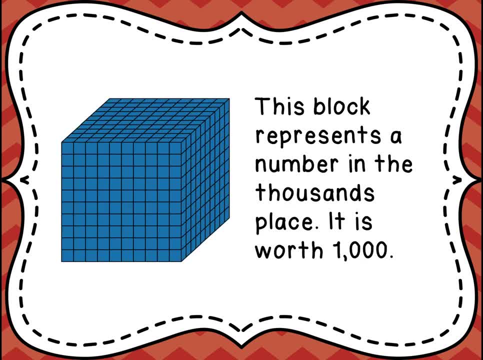 numbers. So here, if you take a look at this screen, you'll see this giant block. This block represents a number in the thousands place, So this particular one is worth 1,000.. If you were to count up all of these little squares, you would see that there are 1,000 of them in this block, This block. 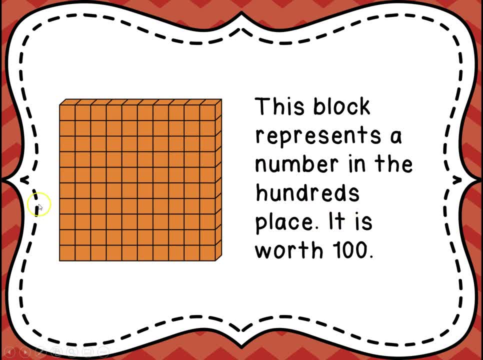 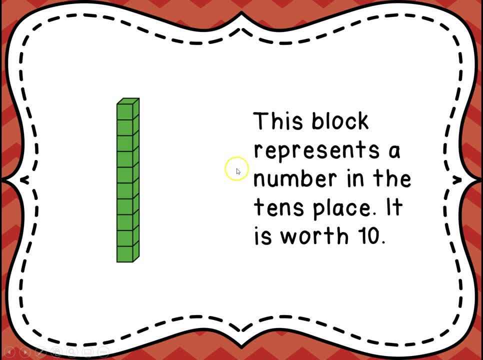 represents a number in the hundreds place. So this particular picture that we're looking at is worth 100.. There are 100 of these squares And this block represents a number in the tens place. It's worth 10, because each one of these rods has 10 squares And this block represents 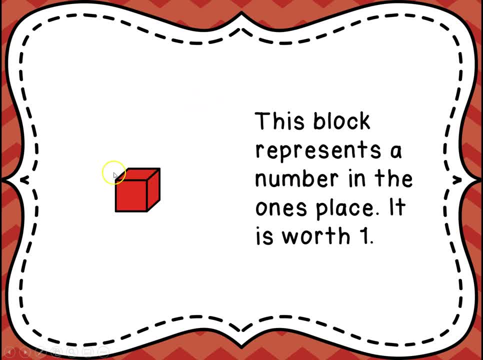 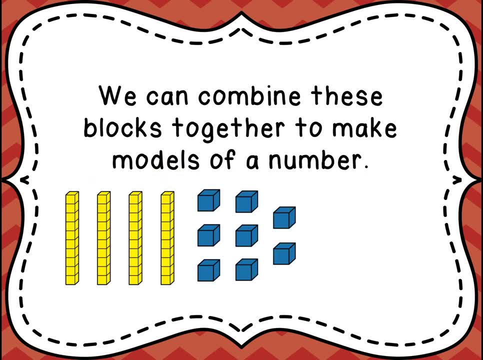 a number in the ones place, It's only worth one because there's only one of these cubes here. Now we can combine these blocks together to make models of a number. So if I take a look I can see that there is one, two, three, four of the tens rods. So we know that there's 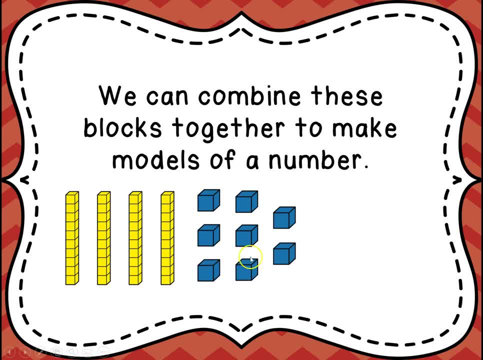 a four in the tens place And there are one, two, three, four of the tens rods And there are 1,, 2,, 3,, 4,, 5,, 6,, 7,, 8.. There are 8 of the ones place. So this model shows the number. 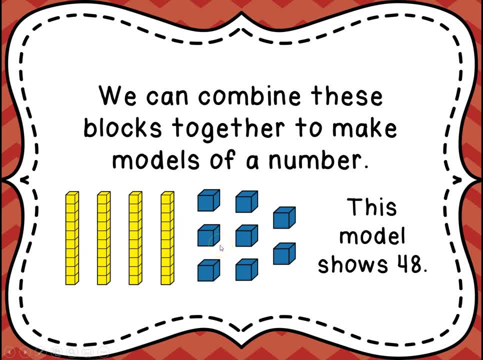 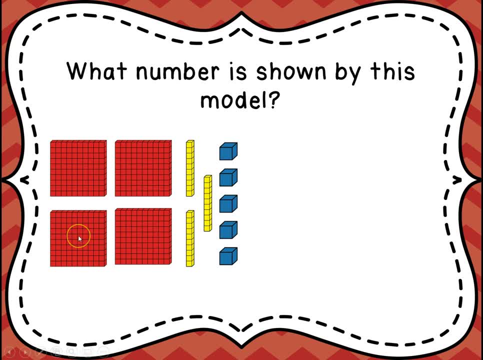 48.. 4 in the tens place, 8 in the ones place. And what number is shown by this model? Well, if you look, you'll see that there are 1, 2, 3, 4 of the hundreds. There are 1, 2, 3. 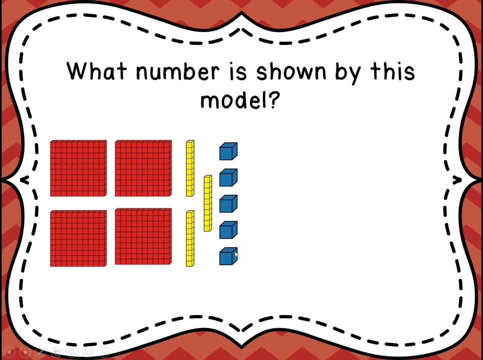 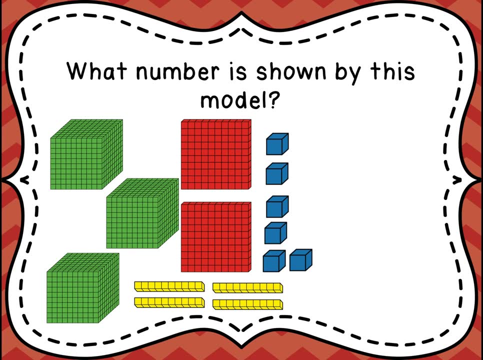 of the tens, And 1,, 2,, 3,, 4, 5 of the ones. So this model shows 435.. You have 4 of the 100's, 400.. 3 of the tens, So 30.. And 1,, 2,, 3,, 4, 5 of the ones, 435.. Now, what model? 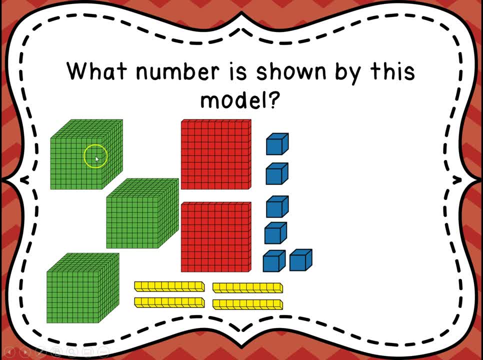 is shown, or what number is shown by this model. Well, again, we're going to count. So we have 1, 2, 3 of the thousands, We have 1, 2 of the hundreds. Here's a number, here's a total, and then another number show you the important juncture. 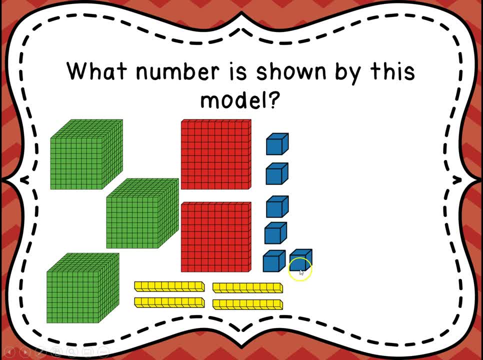 1,, 2,, 3, 4 of the tens and 1,, 2,, 3,, 4,, 5,, 6 of the ones. So we have the number. this model shows: 3,246.. 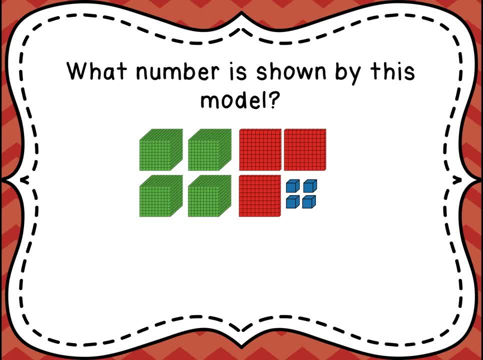 All right, now time for a little quiz. You've got a model on the screen and I want you to tell me what number is shown by this model. So take a moment, count up what you see And then tell me: is it A 3,414,, B 4,310,, C 3,410, or D 4,304?? 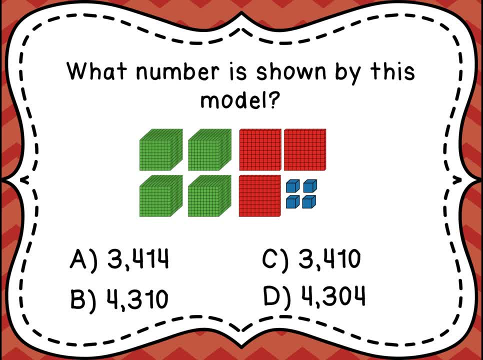 So go ahead and take a moment and count that, see what you come up with. And if you told me that the correct answer was 4,304, because there are four in the thousands place, then you're correct. Three in the hundreds place. no tens- there are no tens rods here- and four in the ones. 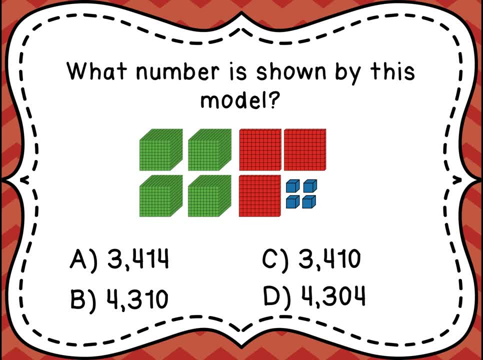 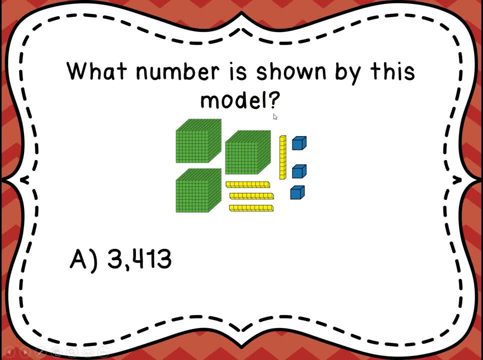 If you said the letter D- 4,304,, you would be correct. Okay, here's another one for you. What number is shown by this model? Is it 3,413?, Is it B 3,013?, Is it C 3,043?? 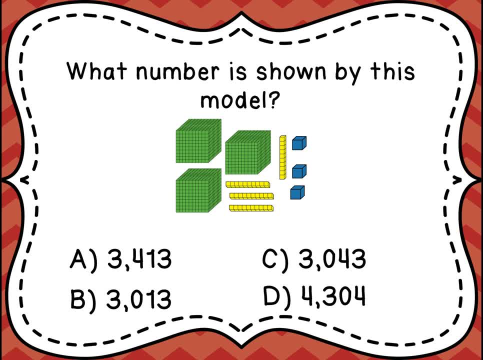 Or is it D 4,013?? Is it B 3,014?? So take a moment and count those up, see how many are in each place, and then you can guess the answer. If you said the answer was 3,043,, you would be correct, because there is three in the thousands place. 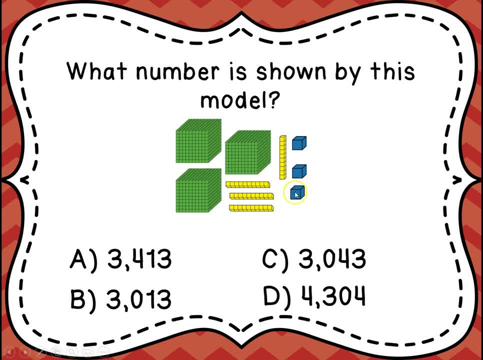 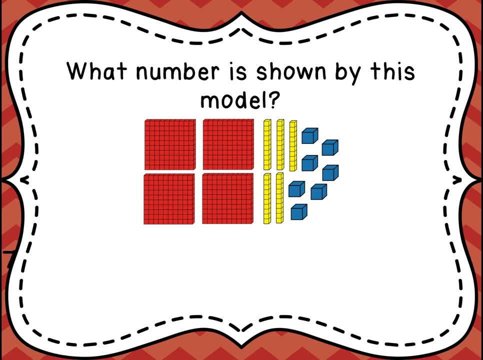 one, two, three, four in the tens place- there are no hundreds here- and one, two, three in the ones: 3,043.. Okay, well, what number is shown by this model? Is it four hundred fifty-seven? 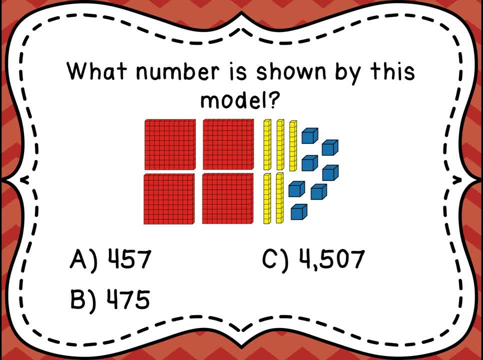 Is it four hundred seventy-five? Is it four thousand five hundred seven Or is it four thousand five hundred seventy? Take a moment, look at the model, Look at each section that's there and then go ahead and choose your answer. If you chose the answer of letter A, four hundred fifty-seven.